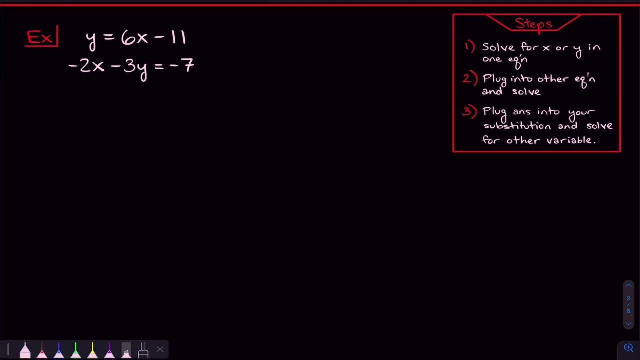 a system of equations with the substitution method. The first step is going to be to solve for x or y in one of these two equations. So let's see, we want to get x or y by itself in one of the equations and, hey look, y is already by itself in the first equation. So that's actually step one. 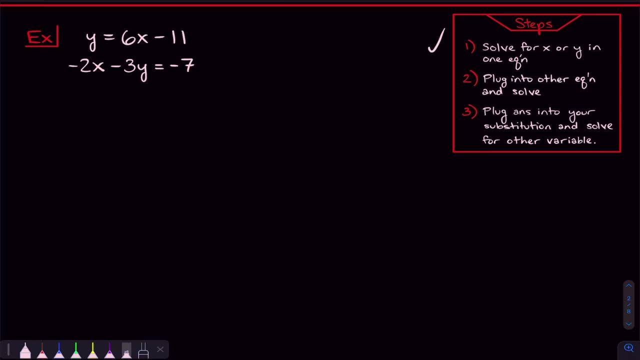 already done. It's already been done for us. So we move on to step two, And step two says: to plug that into the other equation and solve. So what does that mean? Well, if we know that y is equal to 6x minus 11, that means that these two things are exactly the same. And so what? 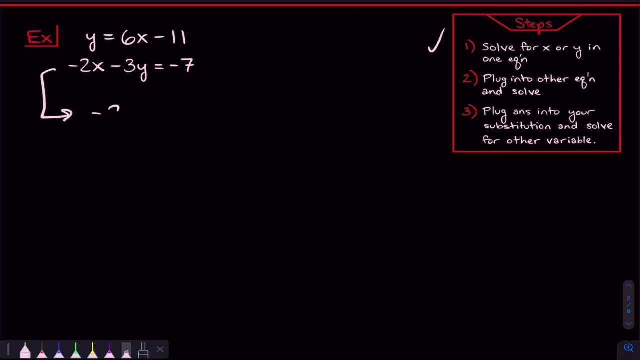 that means is that if I take this other equation right here and I start writing it out, negative 2x minus 3 times y- y we just said- is the same exact thing as 6x minus 11.. We know that because they're. 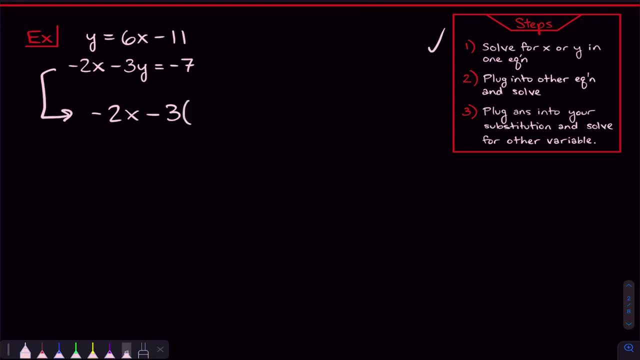 equal. So what I can do here is Plug in a 6x minus 11 for x And then I just continue this equation. it says: equals negative 7.. Now the advantage to doing that is well, that now we don't have any more y's. Before we couldn't. 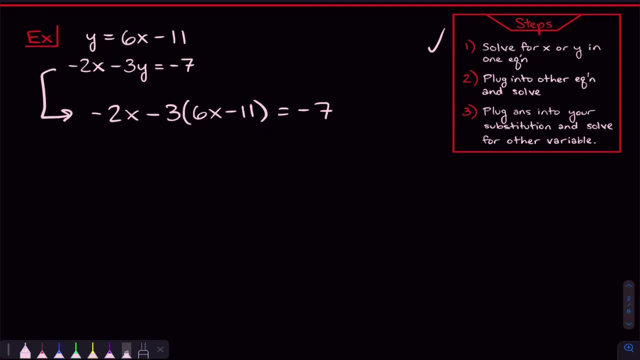 solve and get y or x equal to a number. But now, since all the y's are eliminated, we just have x's left and we can, And you're going to see that right now. So what we're going to need to do is distribute through this negative 3 here. If we distribute that negative 3,. 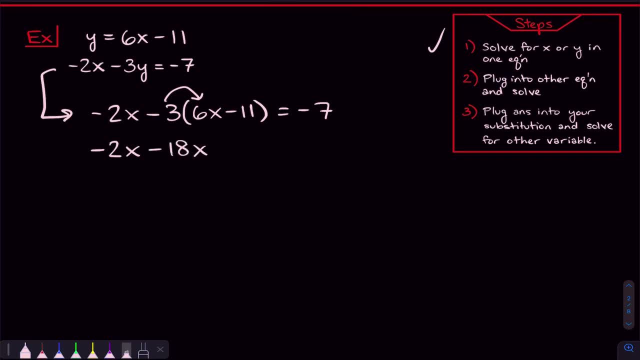 to the 6x, we're going to get negative 18x. That's negative 3 times 6. Then we distribute that negative 3 to the negative 11.. Negative 3 times negative 11 is a positive 33. And that's going to be equal to negative 7.. Okay, so now there's a few things we can do. 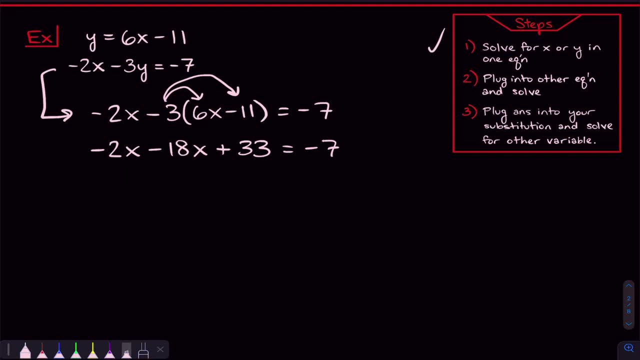 We can combine like terms here to get negative 20x, And also we have a 33 on this side, So that doesn't have an x on it. We want to get that to the other side. We can do that by subtracting. 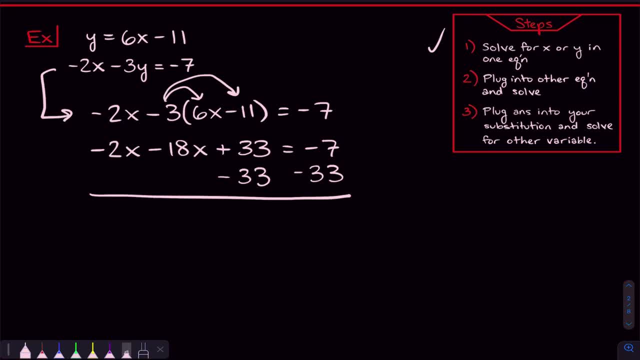 3 on both sides. So we're kind of killing two birds with one stone here. That's something I like to do when I solve this. Hopefully it's not overwhelming for you. So again, combine like terms here: Negative 2x minus 18x is going to be a negative 20x, And then on the other side you're. 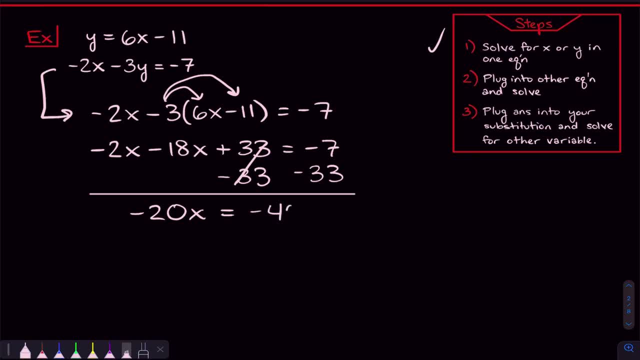 going to get negative 7 minus 33, which is a negative 40. And now, dividing by negative 20 on both sides, we're going to be able to completely solve for x, And negative 40 divided by negative 20 is going to be 2.. So we get: x is equal to 2.. Great, that's one of our variables already solved for. 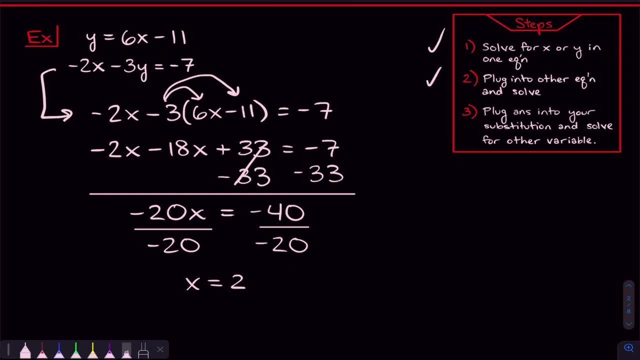 And that completes step two. That's a horrible looking check mark. Let's do that again. There we go, So that moves on. that moves us on to step 3, which says to plug that answer- that x equals 2, into our substitution and solve for the other variable. What's our substitution? Our substitution. 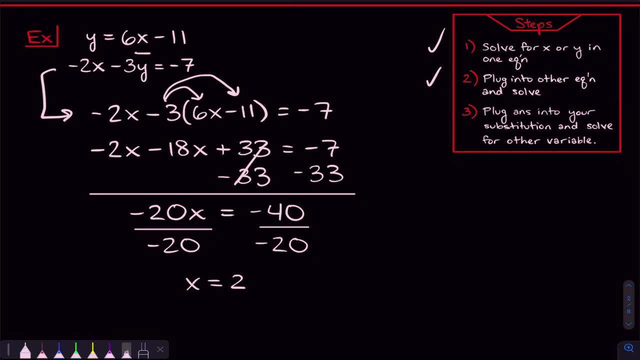 is the equation that we used to substitute. So here we used this equation right here to substitute 6x minus 11 for y. We did that down here. So that's what we want to plug into and that's going to allow us to solve for our. 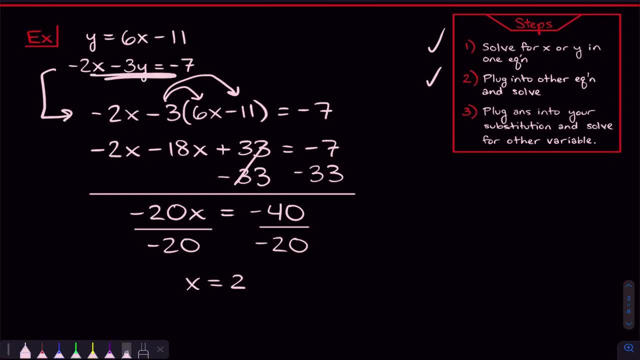 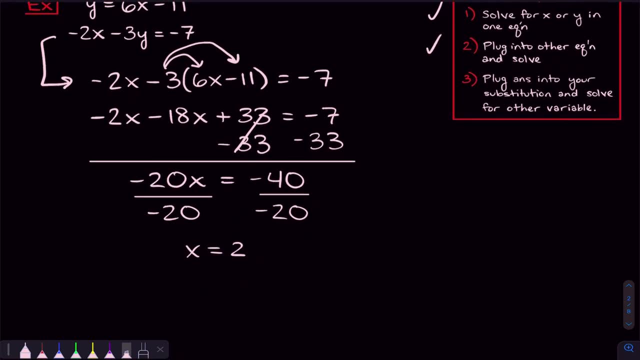 other variable. Now, the reason why I say to plug into our substitution and not the other equation is because this equation is already solved for y, which is now what we want. We want to know the value of y, So that's why plugging into our substitution is so convenient. So here we go. 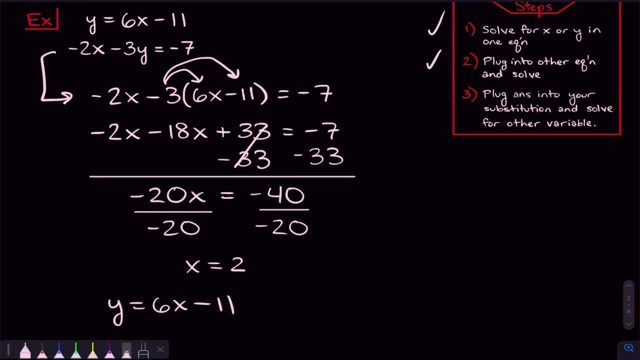 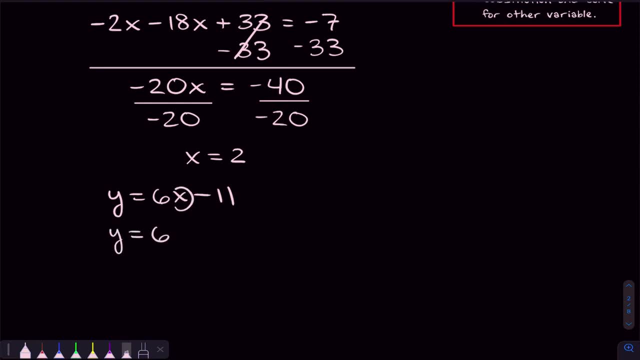 y is equal to 6x minus 11.. That's the substitution that we used, So now we can plug in that x is equal to 2 and solve from there. So x instead of x we're going to have a 2 here. That gives us 6. 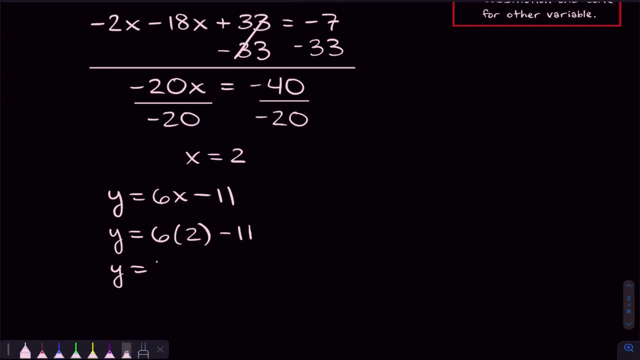 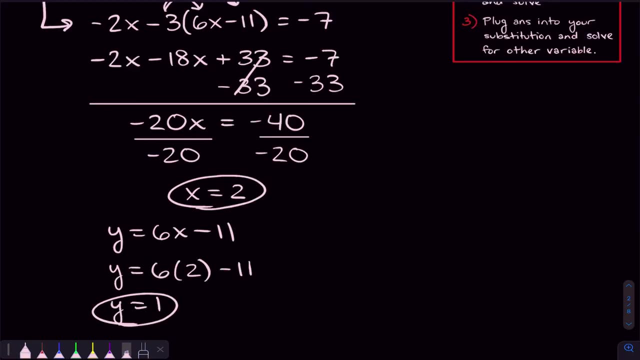 times 2, minus 11.. 6 times 2 is 12.. Minus 11 is going to give us a 1. And right there we have our x, our y. This problem is done. So writing our solution as a point, as a coordinate, as x comma y. 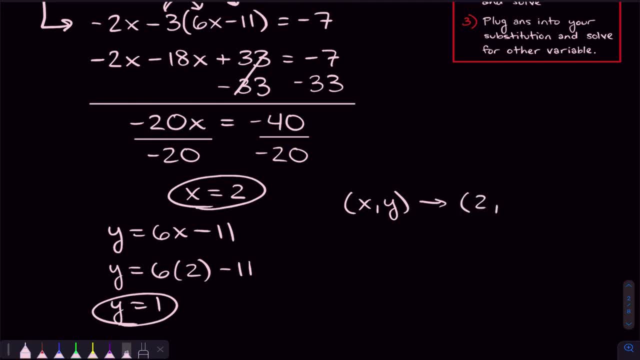 our x is 2 and our y is 1.. So the point here that we get as our answer is 2 comma 1.. So we're going to do plenty more of these examples here, But first, what are we actually finding? Like what? 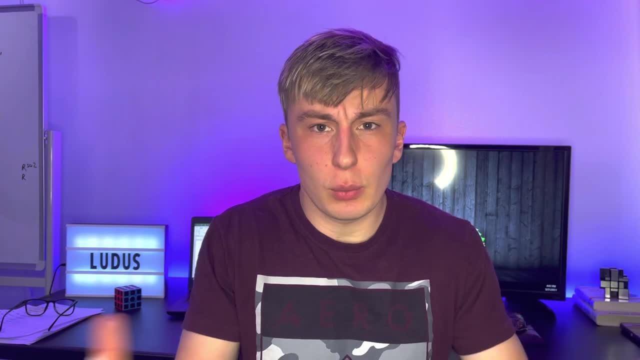 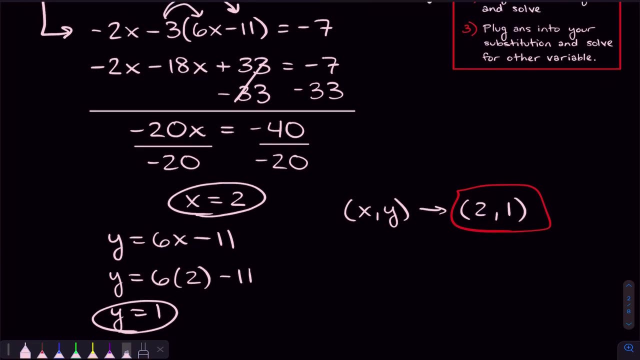 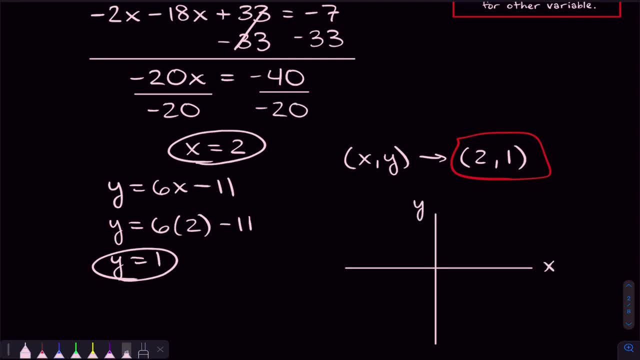 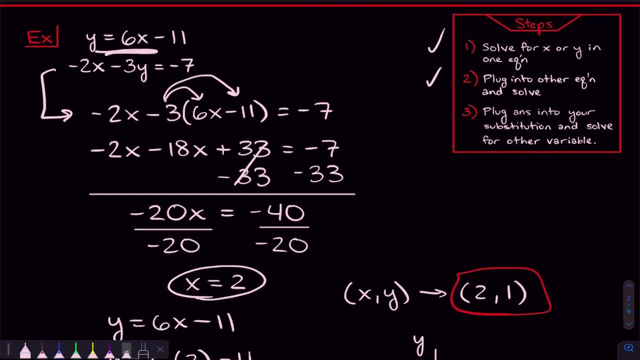 your x- y plane. here I'll draw it out. So here is your x- y axes, And what these two things are is they're lines. This, you can see, is already in: y equals mx plus b4.. It's just going to be some. 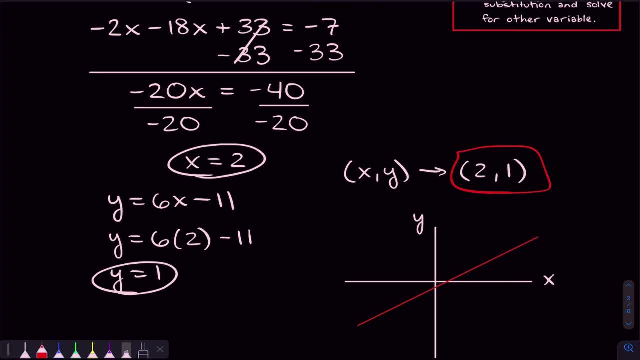 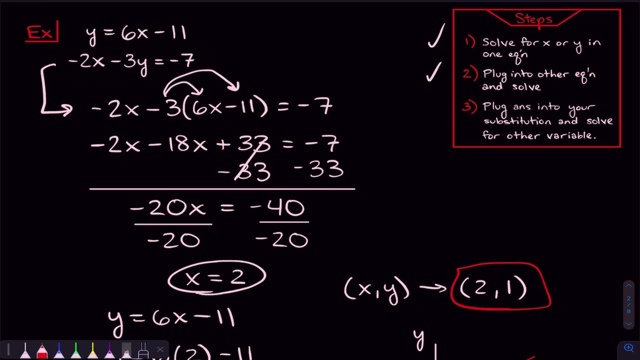 line. I'm not going to draw the exact line here, but let's say it was something like this. And this other thing here. it might be hard to see how it's aligned. This is just another form that you'll commonly see: lines written in with the x and the y on one side and the number without an. x or y on the other side. But if you solve for y, you'll see that it's a line. And if you solve for y, you'll see that it's a line. And if you solve for y, you'll see that it's a line. And if you solve for y. 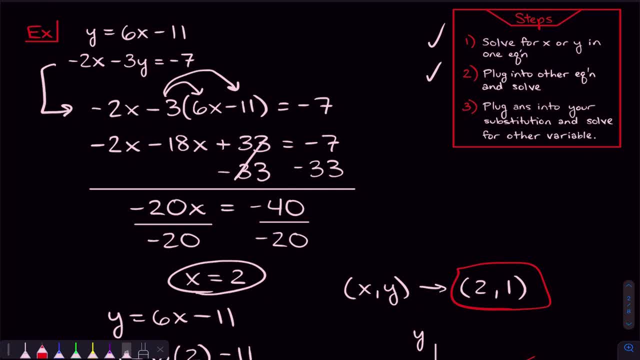 here. you can get that into y equals mx plus b form as well, And you can try that on your own if you like, but just trust me, it will go into y equals mx plus b4.. So this is also a line, And so 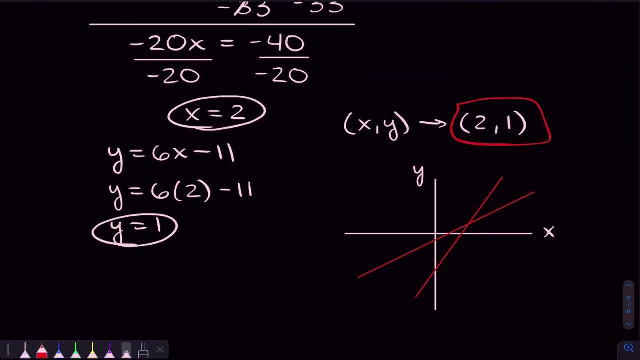 if I graph that line. I'm not going to graph the exact line, But maybe it looks something like that. when you solve a system of equations, what you were finding is where these two lines intersect, And so here I drew the intersection about where it should be. Let's say, this is two over and one up. 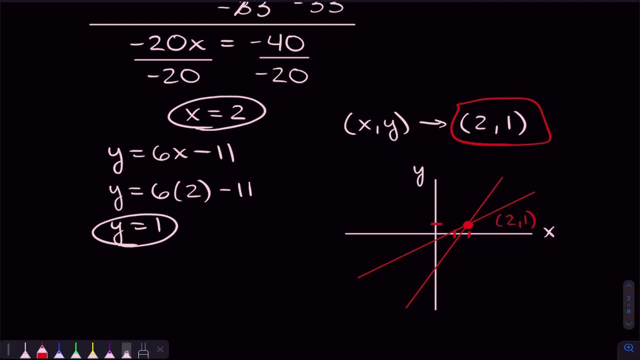 here we found that intersection is at two comma one. that is what you're finding when you solve a system of equations. you're finding where those two lines intersect. So hopefully that helps you understand what we're actually doing here. Moving on to our next problem here Now, this one is: 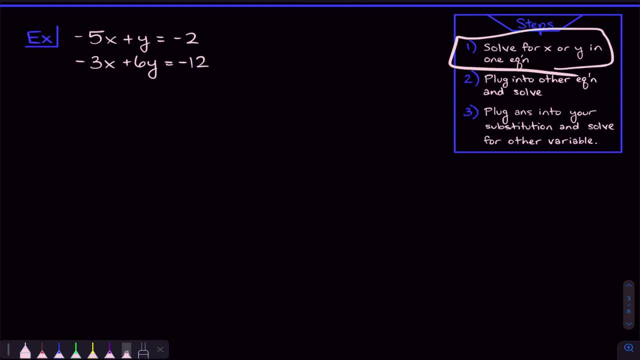 going to require a little bit more work, Because we're actually gonna have to do step one this time. before we already had that y solved for, But now we actually need to solve for either x or y in one of these two equations. Now you can do that in the first equation, you can do that in the second. 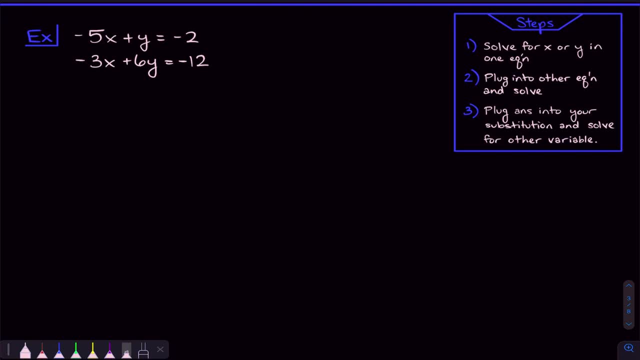 equation. you can solve for x or y. But there is a little bit of strategy to this, Because, if you notice, here this y is already all by itself. there's no number on it. It's not like a two y or a three y, it's just y. And so what I want to do, what I would do, is just solve for y right away. 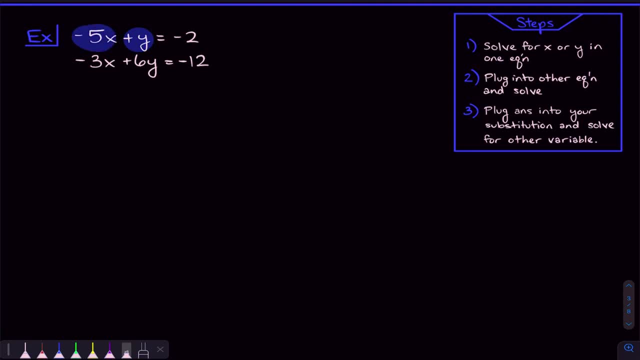 because all you would need to do to solve for y in the top equation is add five x on both sides. So let's do that: If you take negative five x plus y equals negative two and you add five x on both sides, you already solve for y And that's just less work for you to have to do. So we get that y. 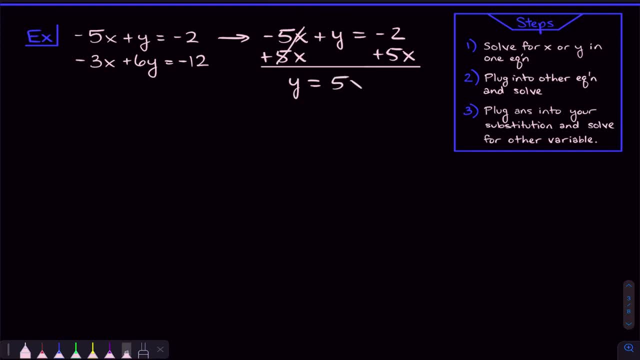 is equal to a five x minus two. Now that is step one completed. we've solved for x or y. we solve for y in one of the equation, And now we move on to step two, which is plugged into the other equation, and solve. So this tells us here that y is the same thing as five x minus two, And so we 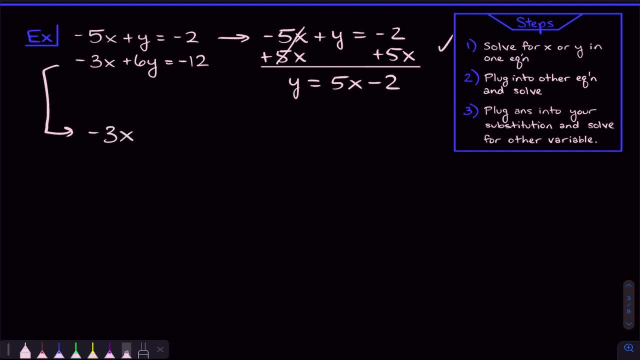 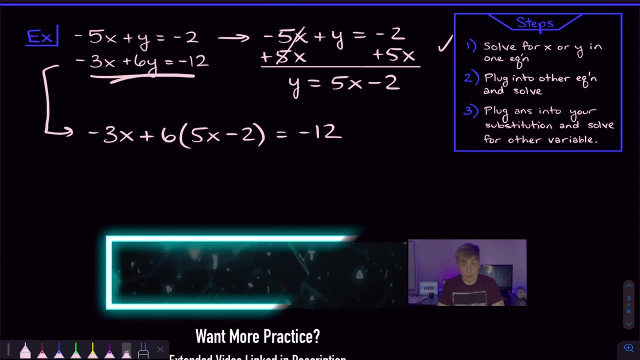 can take this other equation here, the second one, negative: three x plus six times y. we can just say that y is five x minus two, because they're the same thing. So you see, here I just rewrote the second equation, but I plugged. 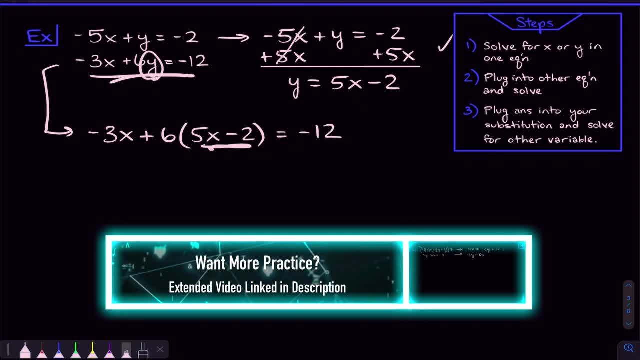 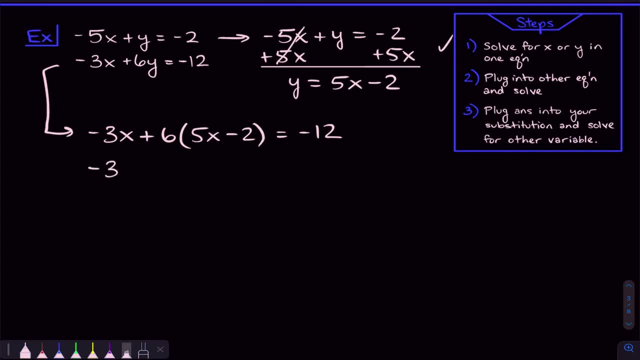 in a five x minus two for y. That's all I did, So now we just need to solve for x. Let's go through and do that. We get negative three x, x. the 6 needs to get distributed through. so 6 times 5x is going to be a 30x, 6. 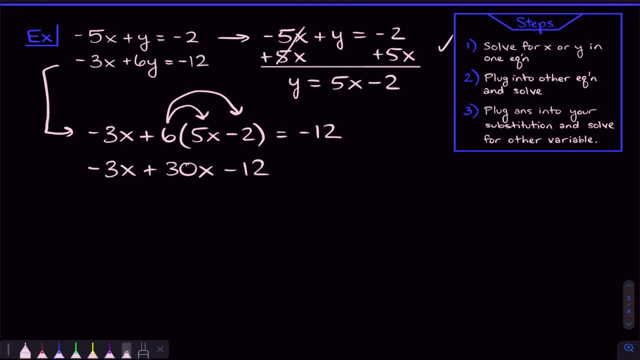 times negative 2 is going to be a negative 12, and then on the other side we have a negative 12. so, as you can see here, with these negative 12s lining up, we're gonna actually get them to cancel because we can add 12 on both sides to. 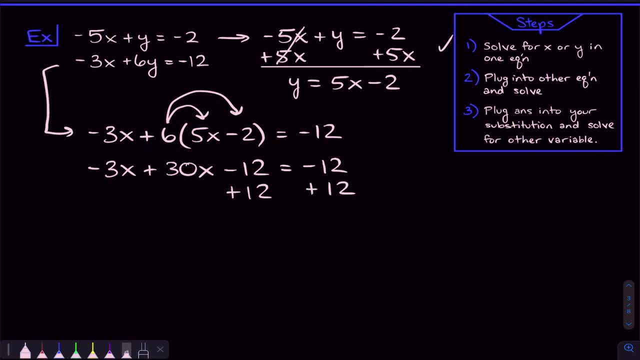 get all of our non X pieces to the right-hand side and what that's gonna do is give us a 0 on the right hand side. then I mean we can just combine like terms here: negative 3x plus 30x, that's gonna be a 27x and you might be able to. 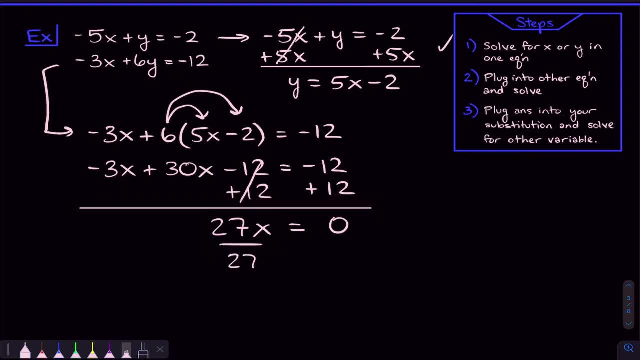 see this already. or, if you want, you can divide by 27 on both sides, but we get that X is equal to 0 and that is step 2 done, so now we just have to do step 3. we got to plug in that answer. we have to plug in the fact that we just found X is. 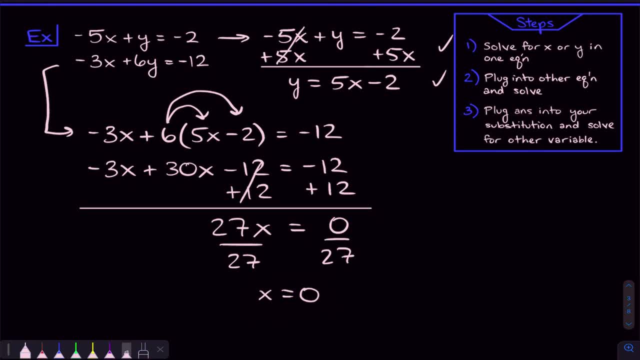 equal to zero, zero into our substitution and solve for the other variable. our substitution is right here and we can plug into that. it's the exact same thing as plugging into our top equation, because this and this are the exact same equation, and i know that because all we did here is we added. 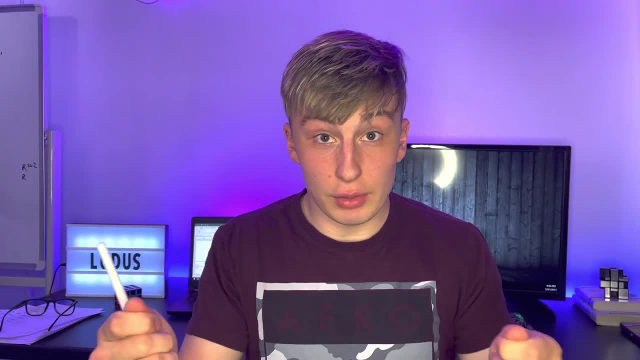 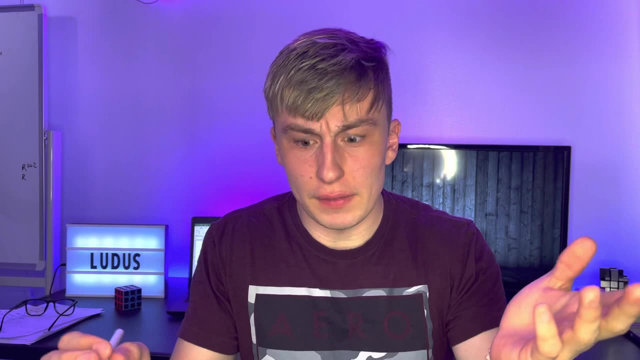 the same thing on both sides. if you do the same thing to both sides of an equation, you're not changing anything. it's still the same equation, it's just in a different form. you know how we can write like you might have done this by now, where you can write lines in different forms. so 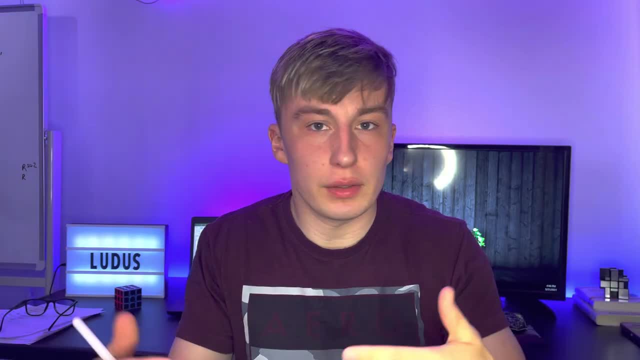 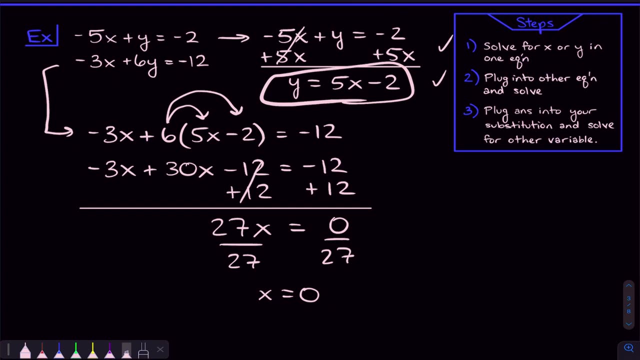 there's like slope intercept and point slope. they're the same equation, they're just in different forms. so, yeah, this is the equation i want to plug into. it's already solved for y, so it's really convenient. so, if i plug into, y is equal to 5x minus 2, which is what that equation. 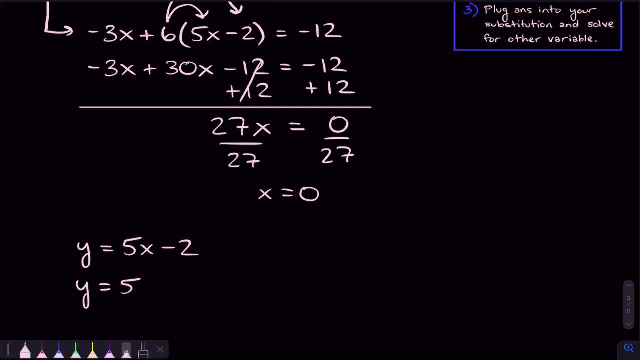 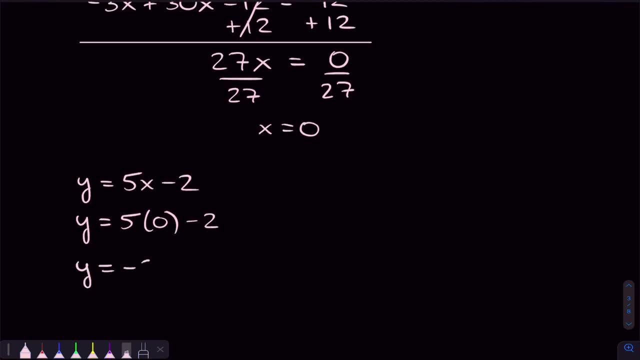 was plug in, the x is equal to 0, which is what we found here. i get that y is equal to negative 2, and now i have my x, i have my y and i can write down what my solution is. where these two lines intersect, my point: x comma y can be written as zero comma, negative two. 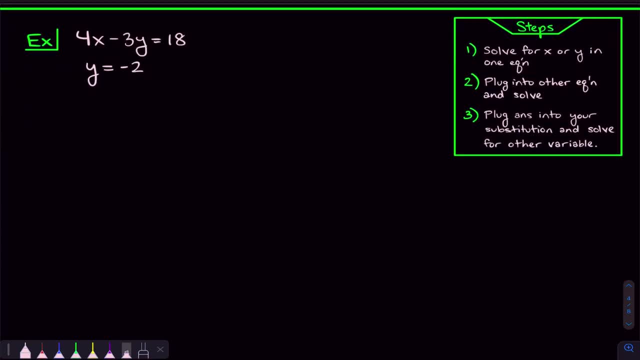 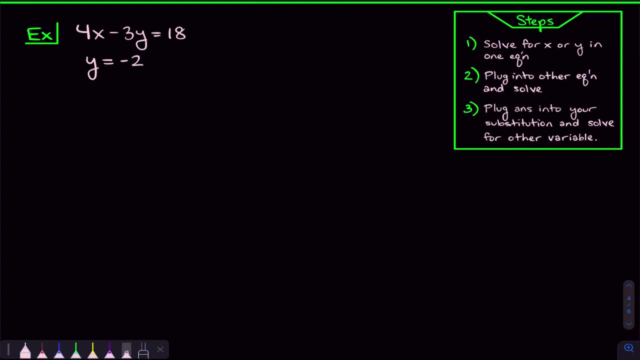 and there we go. so, moving on to our third problem. here we actually afford to do, but this one is very, very quick, and the reason why i wanted to even bring this up in the first place is because people get confused when they see something like y equals negative two. they don't see any x's in that bottom equation and that freaks them out. a. 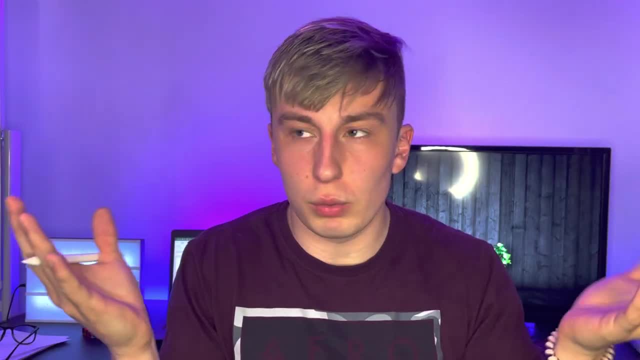 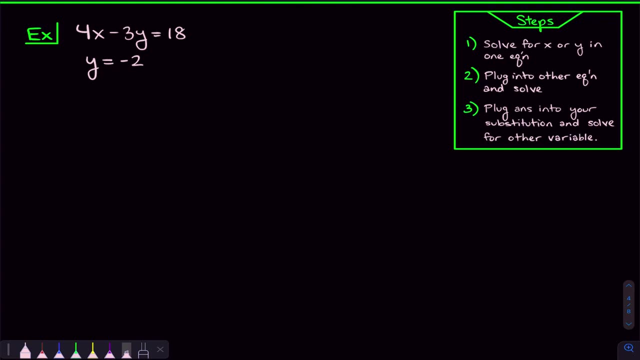 little bit and it definitely freaked me out. when i was in algebra one. i was like: well, what do i even do with that? so here's what you do. let's still follow our step-by-step process. we're going to stay true to it and you'll see how the fact that we don't have any x's here actually 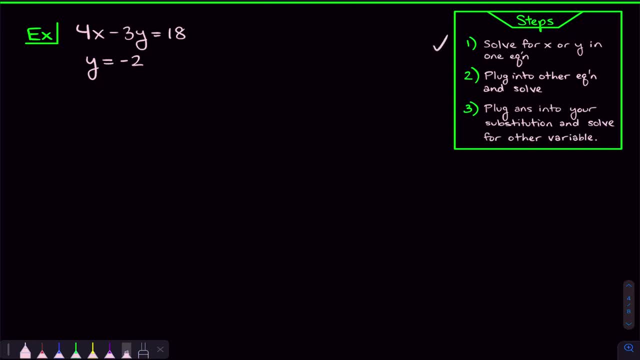 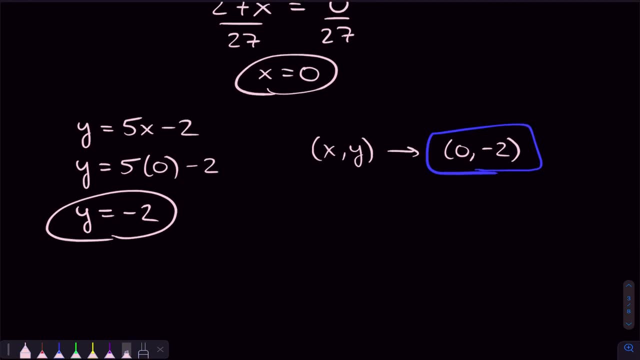 is really nice. so step once is to solve for x or y in one of the equations. that's done. y is solved for right here. and not only is it solved for, but we already have it as a solution. before actually in here, y was equal to negative two. we want to get x or y equal to a number. 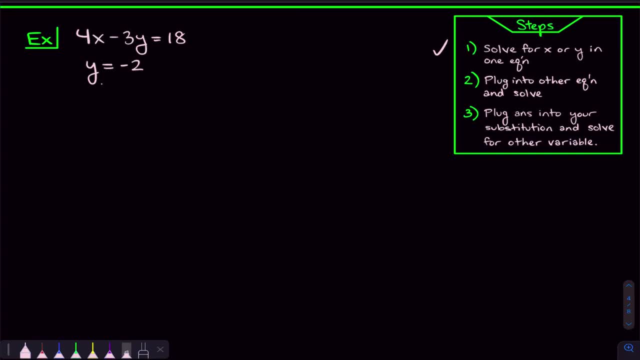 that's our goal, and in this third problem, here it already gives us one of the solutions. it gives us that y is equal to negative two, so now we just need to find what x is equal to, so that that's basically the second step already done for us, because we already have one variable solved for. 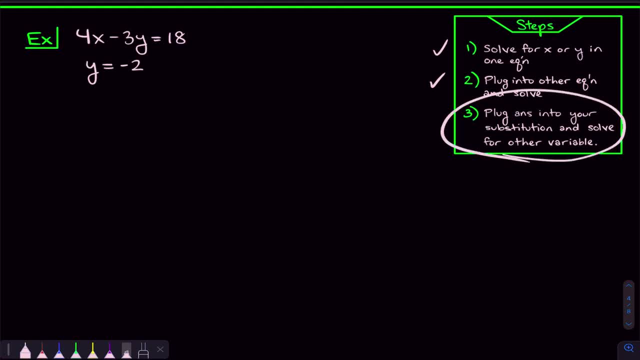 you know. so the only other thing we need to do is plug that answer in to the other equation. we write 4x minus 3 times y, which we know y is negative 2, that's what this equation says, and that's equal to 18.. so let's just solve here 4x. we have a negative 3 times negative 2. that's a positive 6. 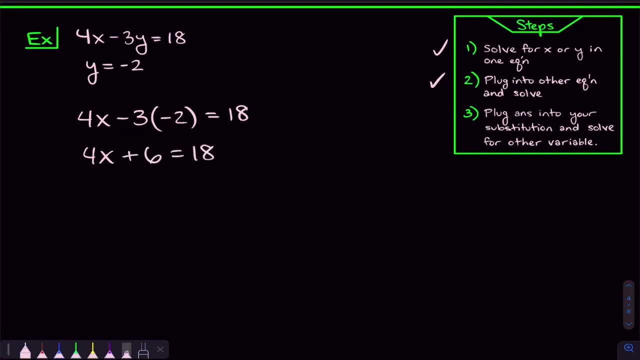 so this will be a plus 6.. and from there, let's subtract 6 on both sides, get 4x is equal to 12, and divide by 4 on both sides to get that x is equal to 3.. so right there we get. x is equal to 3, y is equal to negative 2.. 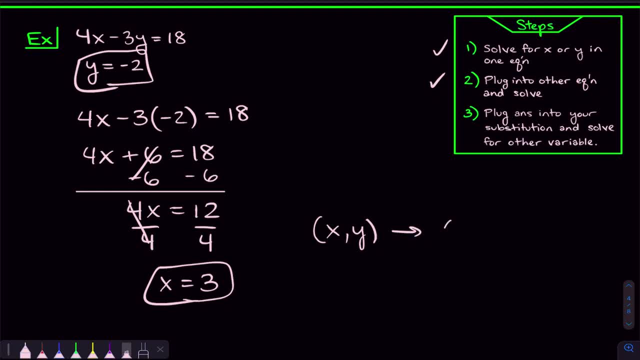 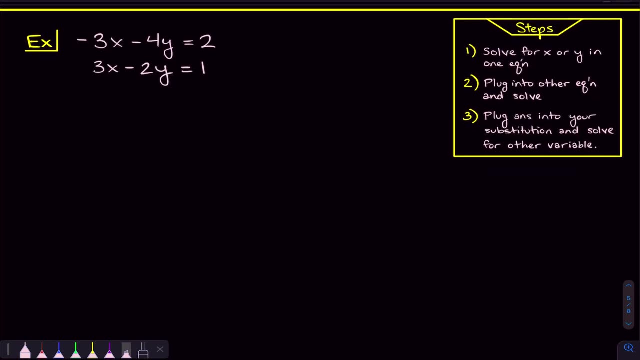 that's our answer. the x- y coordinate pair where they intersect is 3 comma negative 2.. so if you see a problem like that, don't get scared. it's actually a lot easier than you might think. a problem that's not much easier than you might think. this problem can get a little bit. 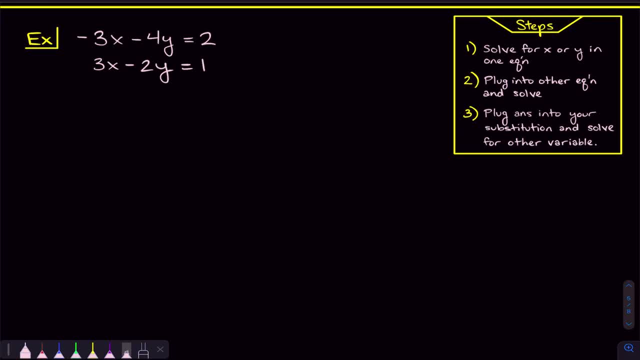 gross because now we're gonna have to do a little bit more work to solve our substitution or to to get our substitution and this problem- if you look to do step one, you want to solve for x or y in one of the equations. now it's not as easy as it was in the second example. 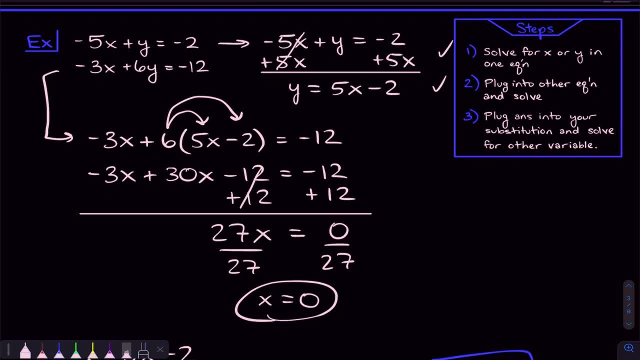 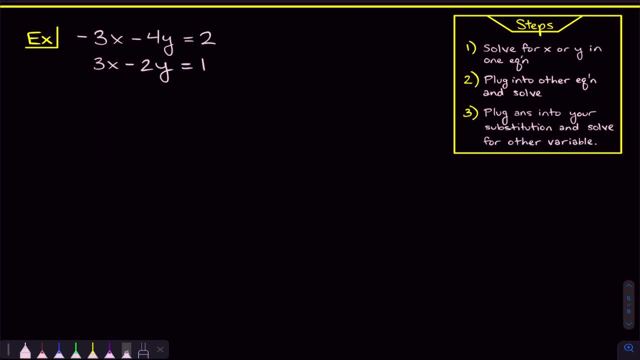 where we saw that y was almost already by itself. so we just wanted to solve for that in this one. they all have numbers in front of them, and so what we're gonna want to do is we're going to just: i would pick for the lowest number, that's what i would do, and 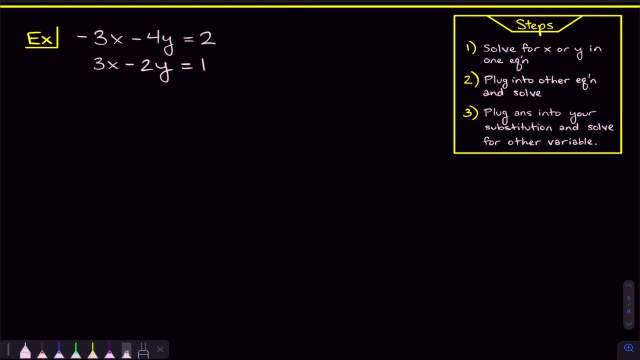 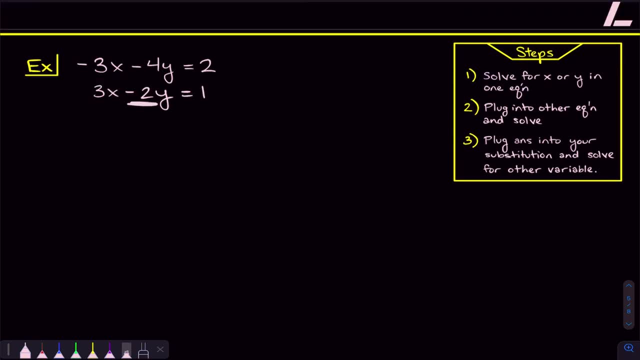 actually i'm going to do that in the bottom equation because it has smaller numbers. i don't want to deal with a four, i'd rather deal with a three, a two and a one. so what i'm going to do here is solve for y in the bottom equation, and i can do that. i'll just take the 3x minus 2y equals. 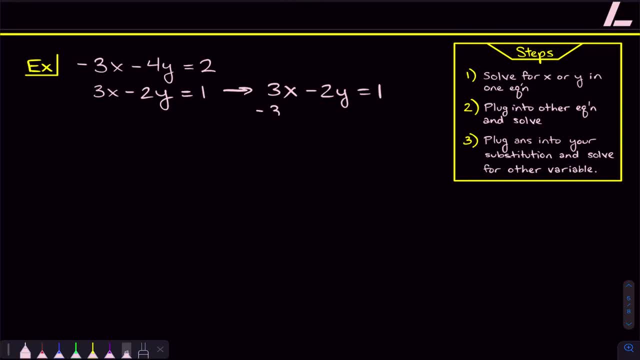 1. i'll put it over here. i'll start by subtracting 3x on both sides to start getting that y by itself. so i get negative. 2y is equal to. you can write this as 1 minus 3x. there's nothing wrong with it. 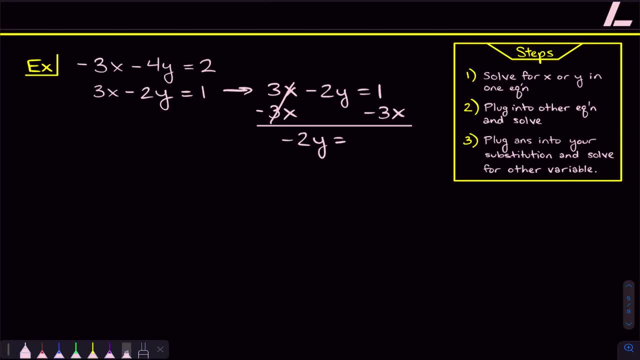 i always like seeing things more in like y equals mx plus b form, so i like to write it as negative: 3x plus 1.. and this and 1 minus 3x are the same thing. that's just the commutative property. so 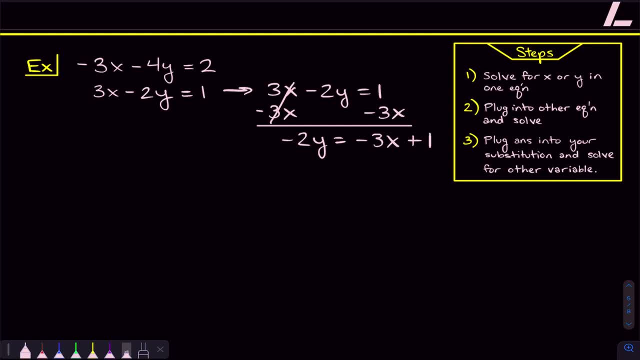 i'm going to write it as negative 3x plus 1.. now we just need to divide by negative 2 on both sides, and if we want to divide this entire thing by negative 2, it's the same thing as dividing each piece by negative 2.. so this is going to become y equal to. we have two negatives. 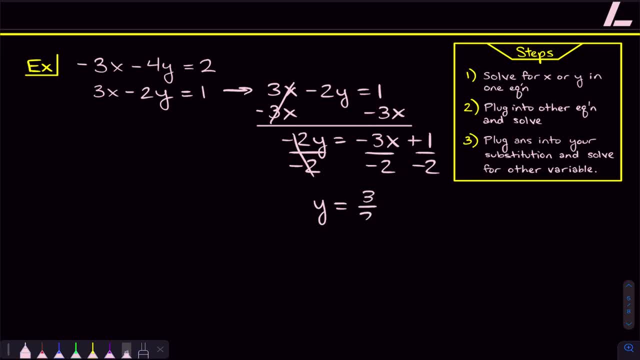 here, and a negative divided by a negative is a positive. so this is going to be a 3 halves x, or you could write that as 3x over 2. it's the same thing. and then this is a negative one half. so that's step one done. we've solved for x or y in one of the equations. we solved for y in the. 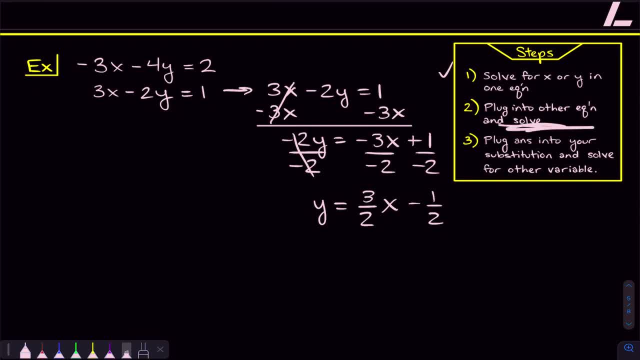 bottom equation. now we need to plug that into the other equation and solve. that's step two. so plugging into the top equation, which is the other one, we know that y is the same thing as three halves, x minus one half. so when we start writing this equation we get to the y part, we get minus. 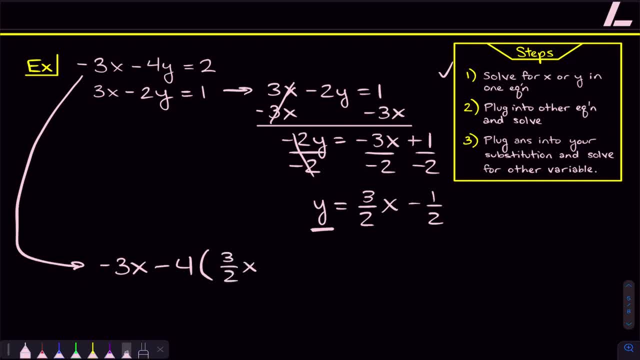 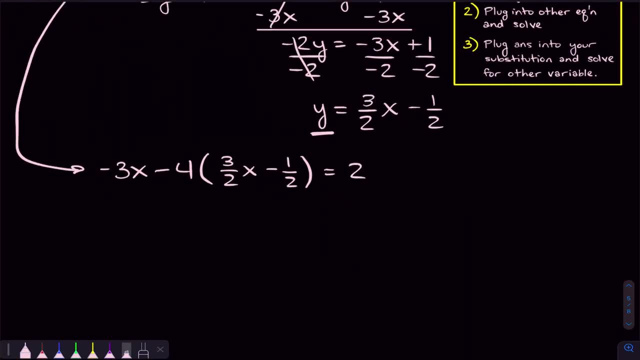 four times y. we can replace that with a three halves x minus one half and that's equal to two. now we just distribute through. so we distribute through that negative four. negative four times three halves. well, that four is going to become a two. this will become a one. 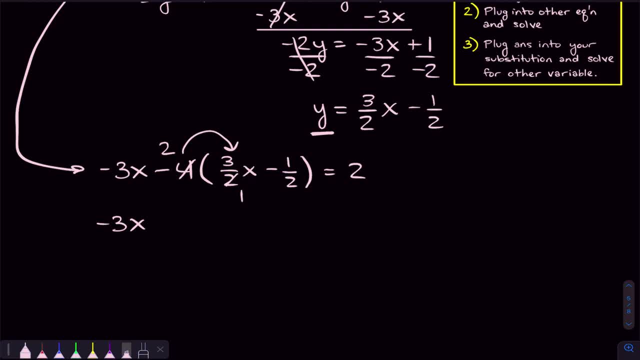 so we get negative two times three, which is negative six, and there's an x there, so it's negative six: x. so that is the first one done and now i'll reset that so we can distribute through the second time. we have negative four times negative one half, which that'll be a positive number, because 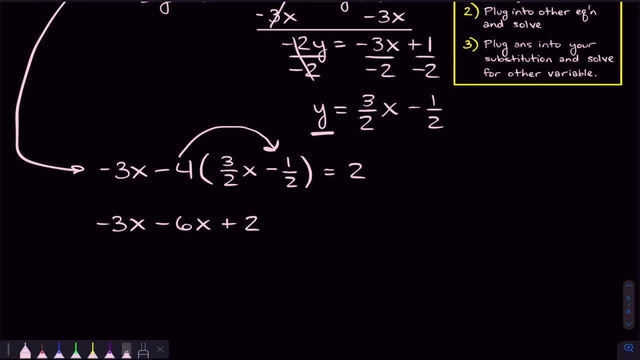 there's two negatives and that'll just be two right, because four divided by two is two and that's equal to two. so now i'm going to subtract two on both sides. so i'm going to subtract two on both sides to get all my non-x pieces to the other side and i can combine like terms over on the left. 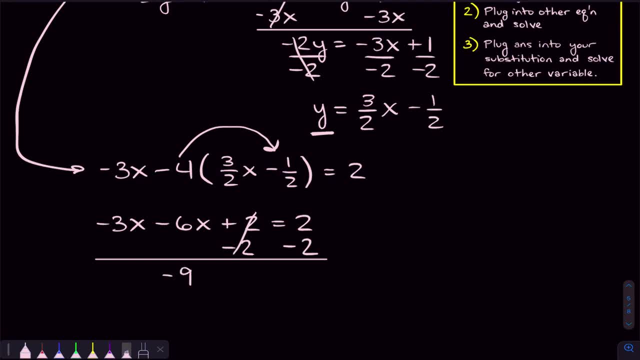 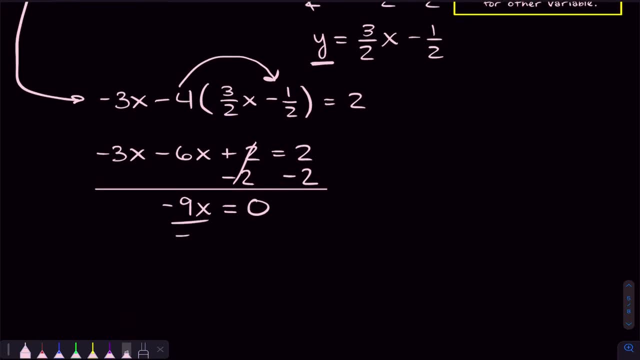 hand side. so over on the left side i have negative 3x minus 6x, which is a negative 9x, and then i have a 2 minus 2 on the right hand side, which is a zero, and as you can see, here we're going to get. 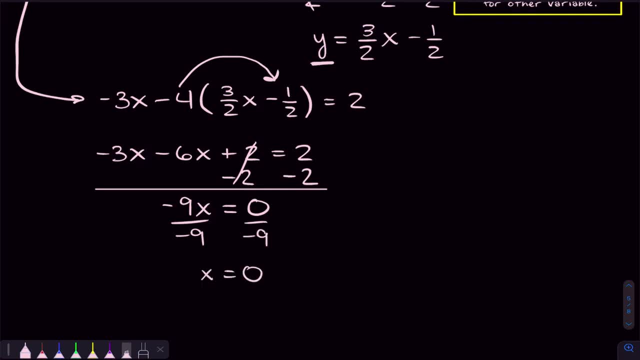 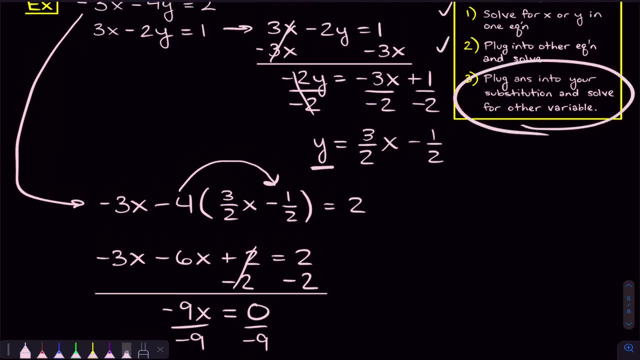 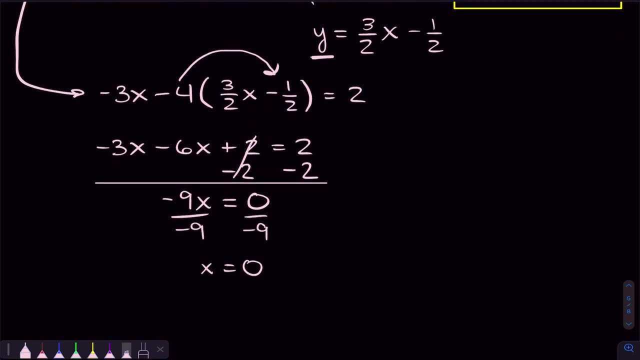 that x is equal to zero. so that's my first variable. solve for that's step two. step three says to plug that answer into the substitution and solve for the other variable. this is my substitution, that's what i'm plugging in for. so again, that substitution is: y is equal to three halves x. 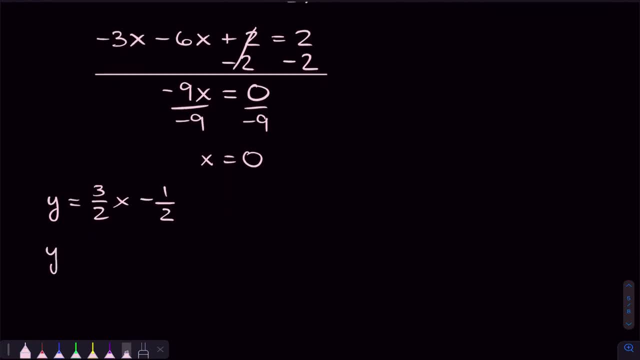 minus one half. and if i plug in that x is equal to zero, then what i'm going to get is that y is equal to this is entire, that that entire thing is zero. so it's just negative one half. so i take this, i take this and those are my answers. so 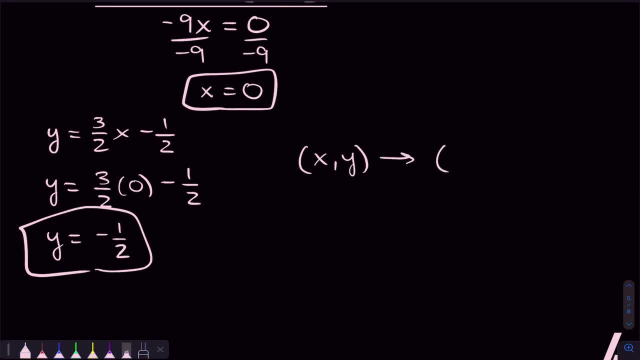 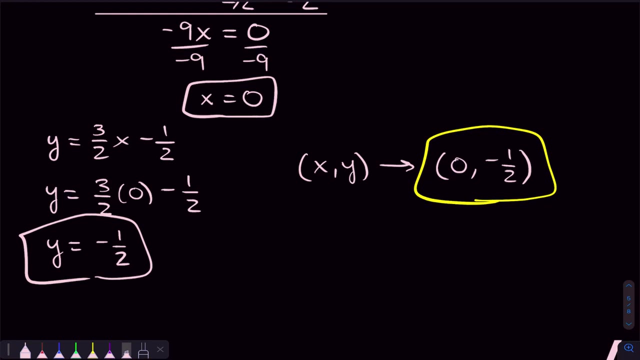 the point of intersection, the x- y pair is going to be zero comma negative one half. and that is the answer for the last problem that we're going to do together in this video, and that's how to solve systems of equations using the substitution method. and, assuming that you feel pretty good with that, here is a problem for you to try. 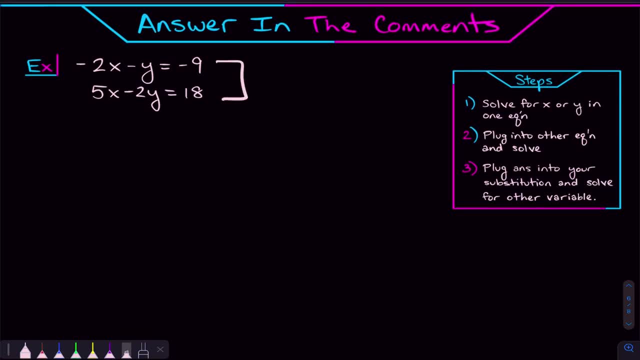 and answer in the comments. so i have another system of equations right here. just follow this step-by-step process, like we've been doing in the four problems that we did in this video, and let me know what your answer is in the comments and if you had any questions on anything. 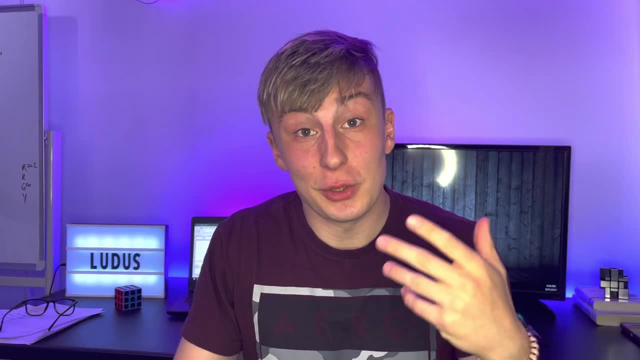 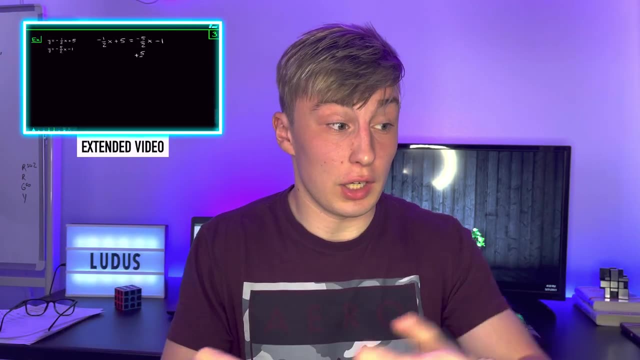 we talked about in this video. again, let me know in the comments and i'll try to get back to you when i can. now again, i have an extra video where we go through 10 more of the systems of equations problems. right in the description we're going to talk about substitution method. 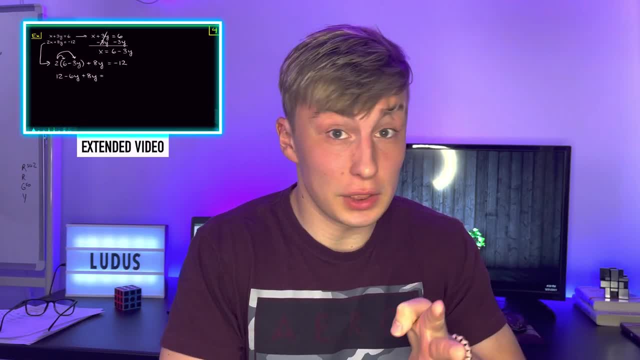 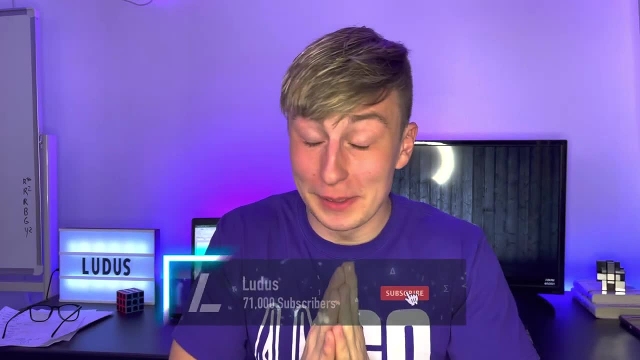 elimination method. we'll go through where we have one solution, no solutions, infinite solutions. we're going to go through all of that stuff, and so that is right in that extra video in the description. lastly, make sure that you're subscribed to this youtube channel. look, i've been recording a lot of. 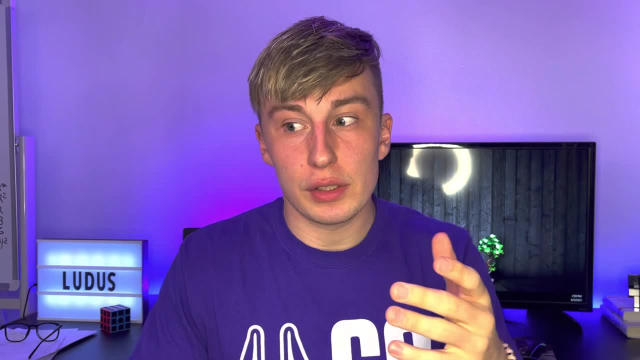 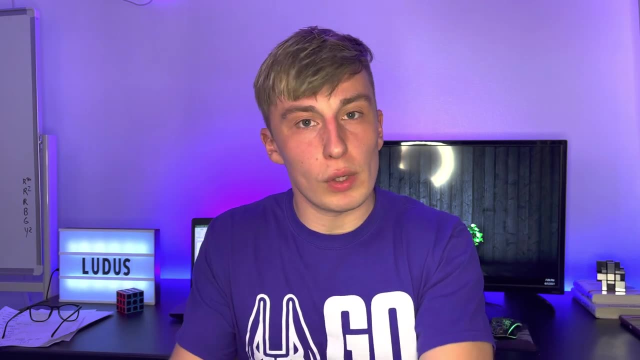 videos today. i've been recording a lot of videos for the past few days for you guys, and so my throat is starting to hurt because i'm talking for literally hours at a time. so what i need you guys to do is subscribe, because if i wasn't poor right now, i'd be able to afford ice cream to like you. 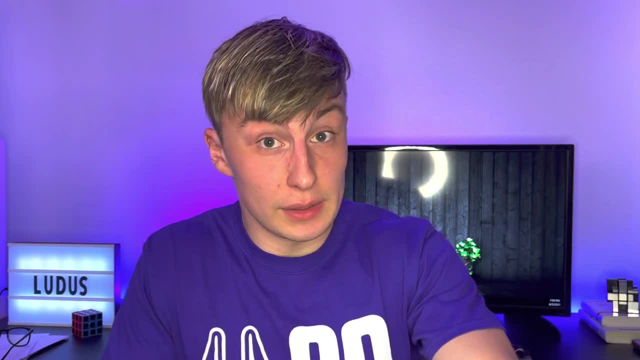 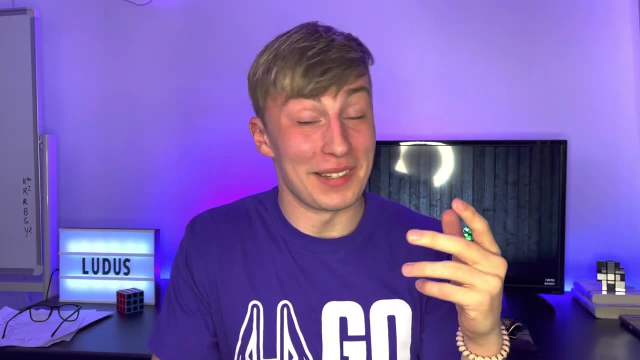 know, help my throat a little bit. so that's what i need you guys to do: help me not be poor, so i can not hurt. okay, with that being said, that's gonna do it for this video and i'll see you guys soon.